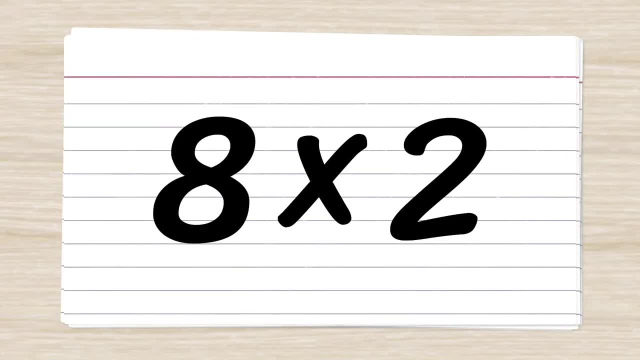 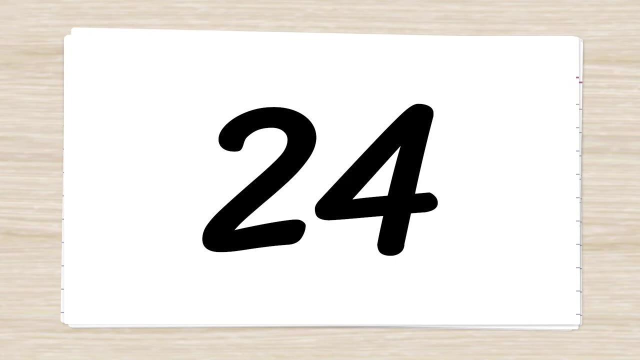 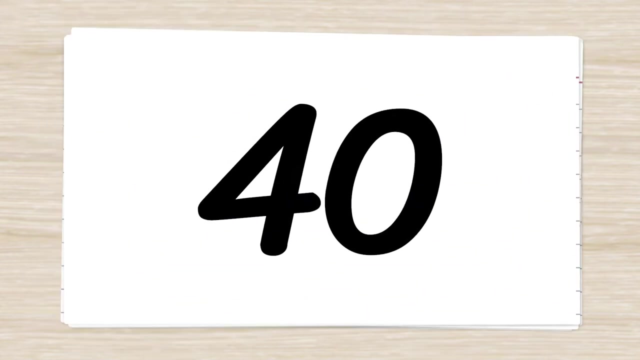 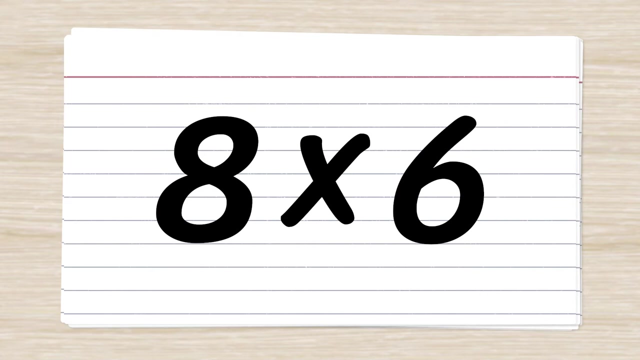 Eight times two. Sixteen Eight times three. Twenty-four Eight times four. Thirty-two Eight times five. Forty Eight times six. Forty-eight Eight times seven. Fifty-six Eight times eight. Sixty-four Eight times nine. 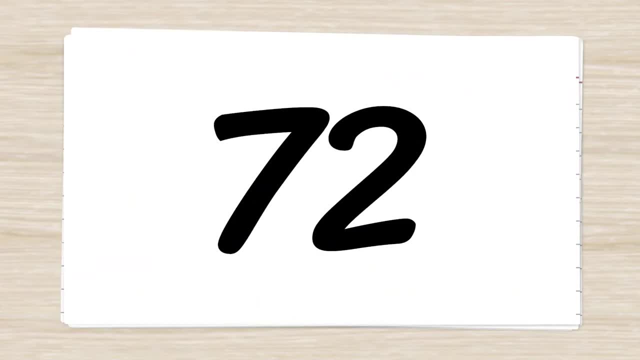 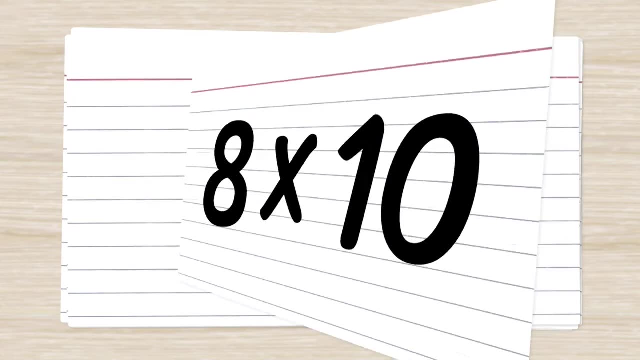 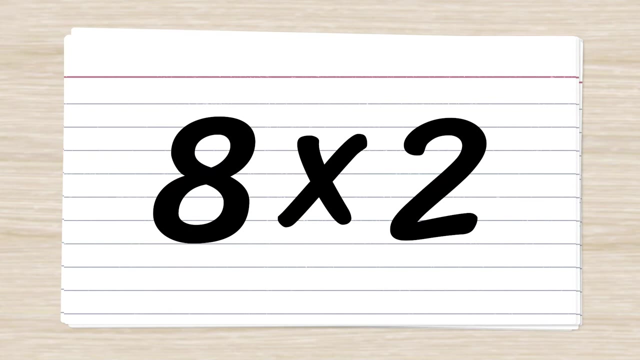 Seventy-two. Seventy-two, Eight times ten. Eighty Eight times two. Sixteen, Eight times nine. Seventy-two, 8 times 1, 8.. 8 times 5, 40.. 8 times 3, 24.. 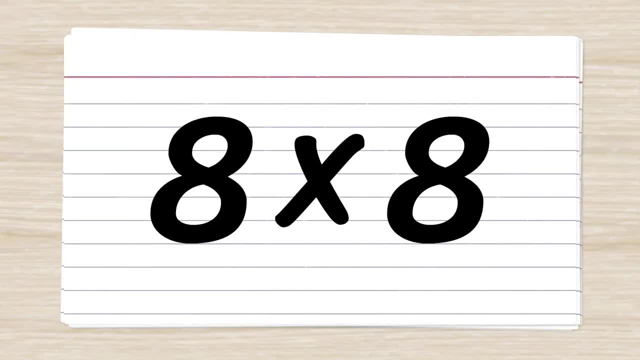 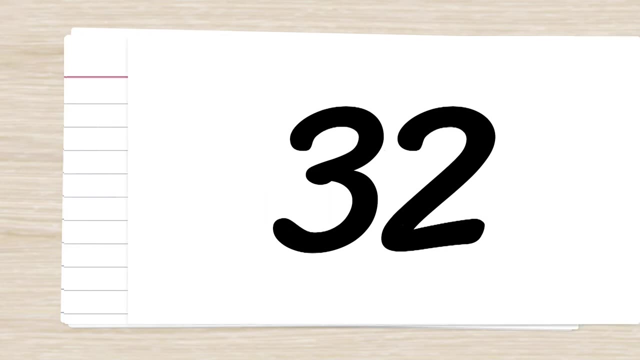 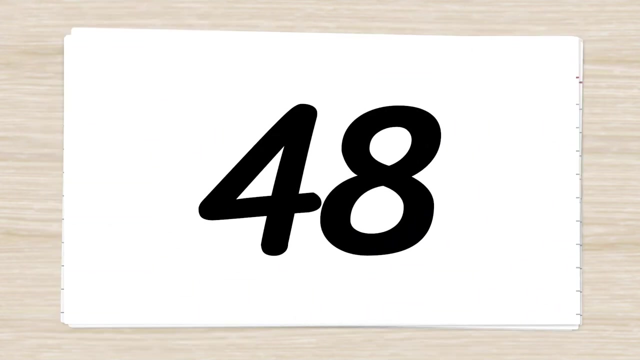 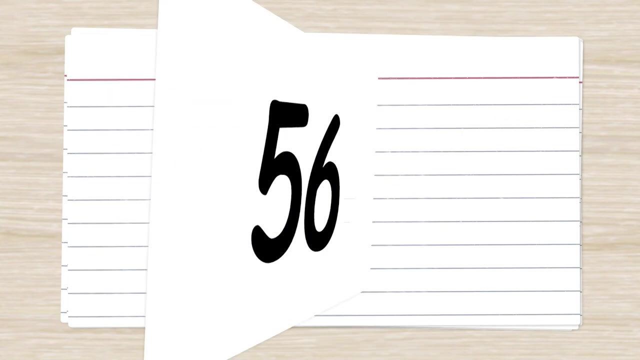 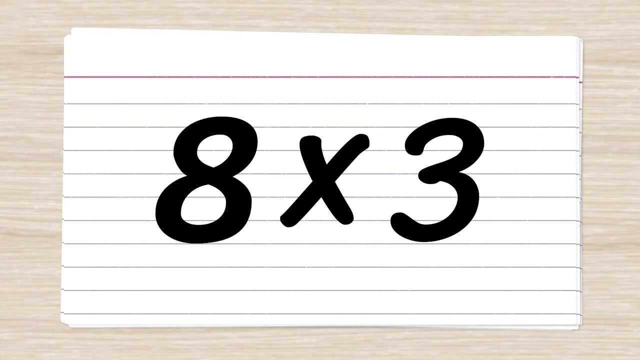 8 times 8, 64.. 8 times 4, 32.. 8 times 6, 48.. 8 times 10.. 80.. 8 times 7, 56.. 8 times 3, 24.. 8 times 5, 40..